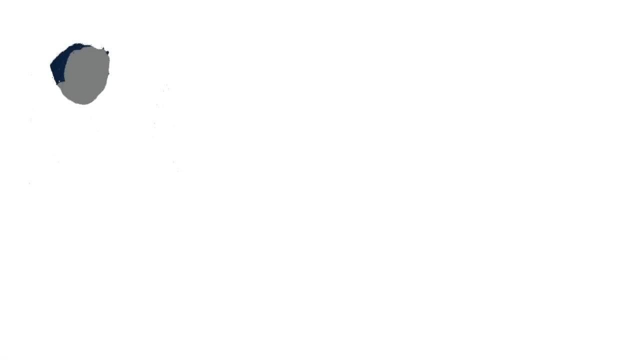 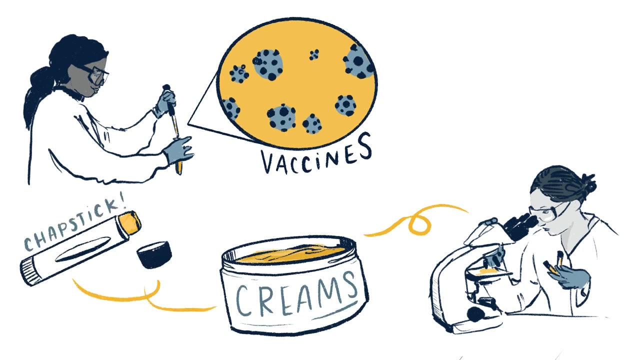 can I create medicines to heal people? Synthetic biologists work day and night to find cures for diseases like COVID-19.. They develop vaccines to protect us all from infection. Some bioengineers may even work for beauty companies inventing creams to soothe your skin or chapstick to 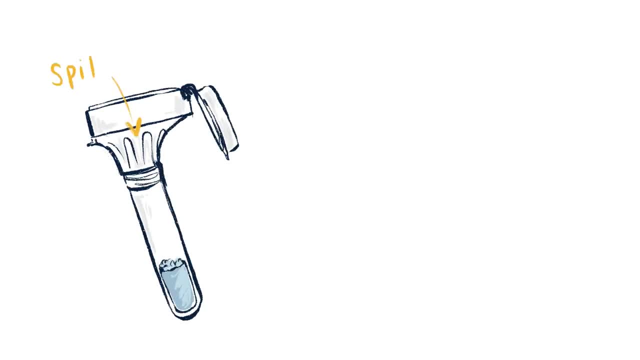 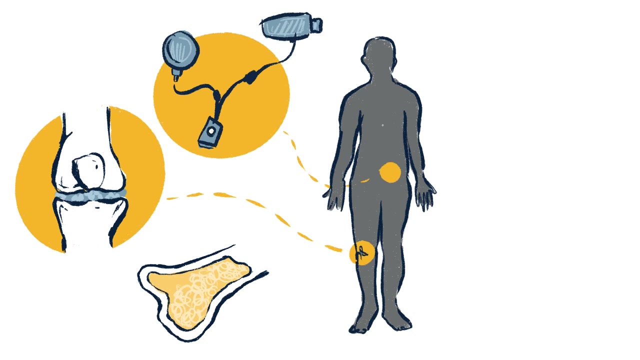 moisturize your lips? And have you ever taken a DNA test to learn more about your family's ancestry? Bioengineers made that possible. How can I grow cells to cure people? Bioengineers can grow artificial bladders, knee cartilage and bone marrow using real cells. 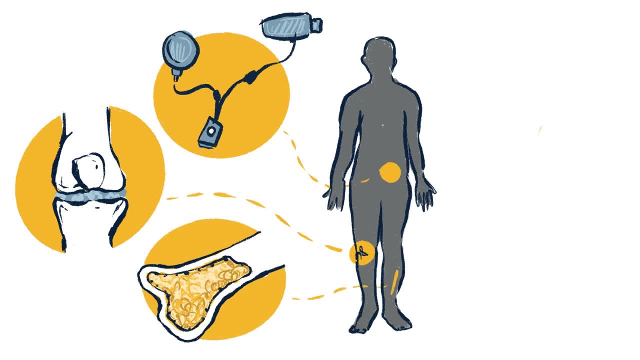 Many patients have received these new body parts to replace their own. Some bioengineers dream that one day we'll be able to grow a human heart in a laboratory, giving new life to people whose hearts are failing. Cell and tissue bioengineers have also grown meat in labs as a new source of food. 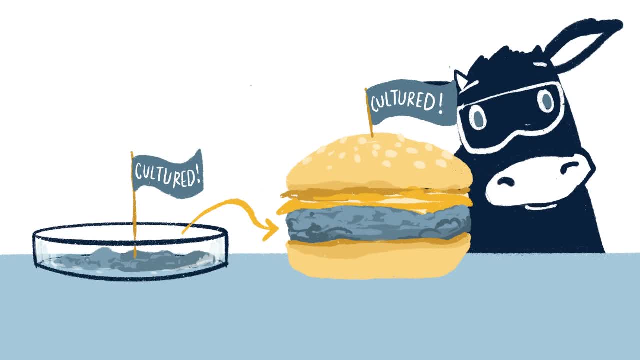 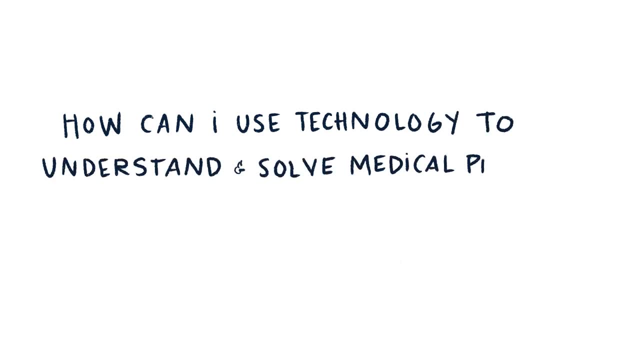 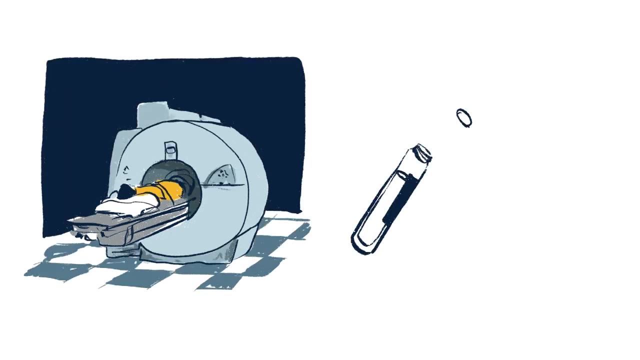 Their cultured burgers taste close to real beef patties and someday might even cost less. How can I use technology to understand and solve medical problems? Biomedical engineers build devices like MRIs and CAT scans. They also developed spit and nasal swab tests that you might have seen to check for coronavirus. Do you know anyone with diabetes? 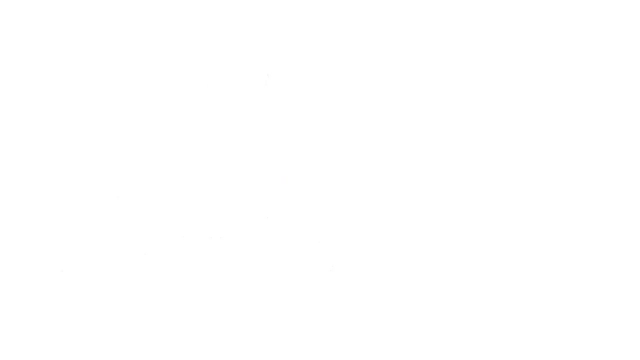 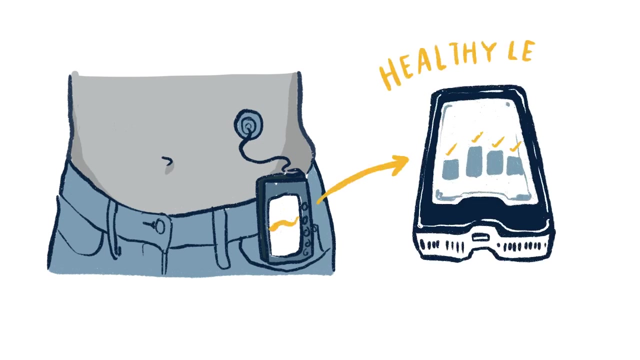 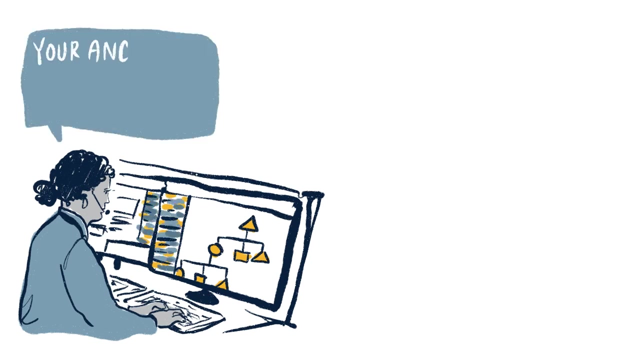 Then you might know that they have to constantly check their insulin level. Biomedical engineers invented a device that measures this, and they even made a pump that automatically helps diabetic patients maintain healthy levels. Some bioengineers use powerful computers to crack our genetic code. They've even taught computers how to measure blood pressure and 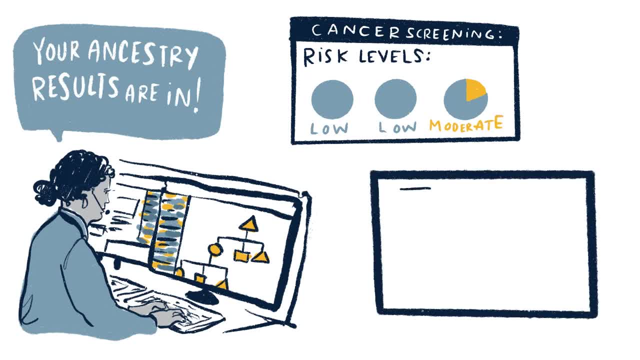 blood pressure levels. Some bioengineers use computers to detect cancer sooner than human doctors. Others track and predict the spread of diseases, like COVID-19,, helping governments decide when we need to stay home and when we can come out again safely. Bioengineers- 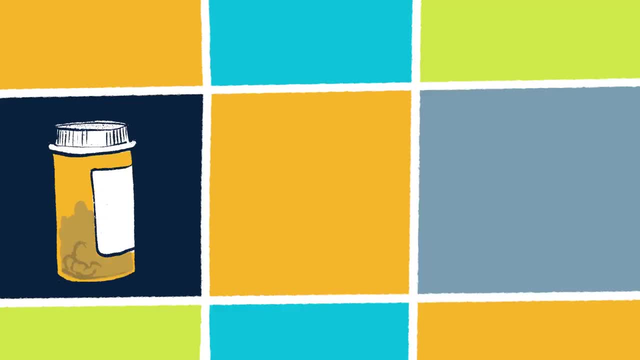 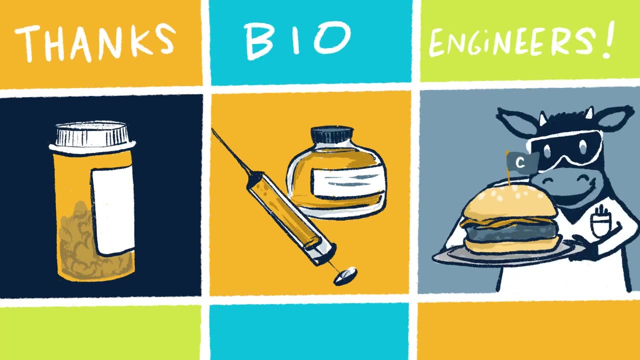 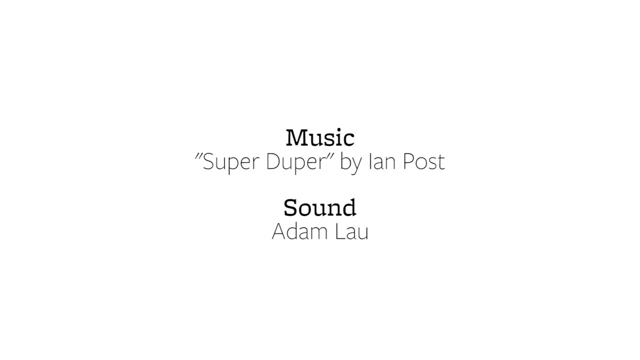 work around the clock to keep us healthy. So the next time you take medicine, get your shots, or perhaps bite into a juicy lab-grown burger. you can thank a bioengineer.